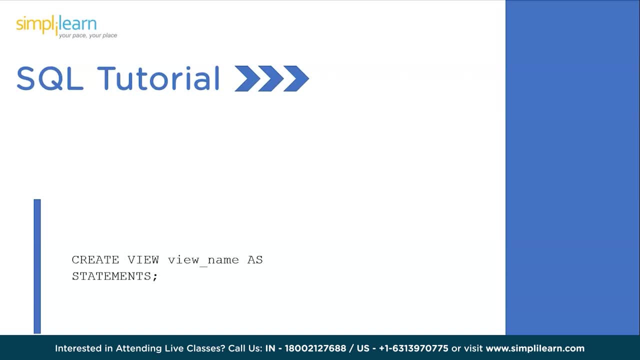 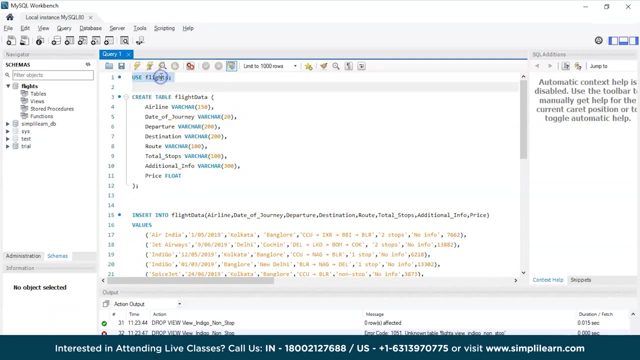 every single time. So if you create a view for that and if you just select that particular view and you get all the data Now let's understand this more easily by going through a practical demonstration on mySQL. Now we are on the mySQL workbench. We are having a small database which is flights. 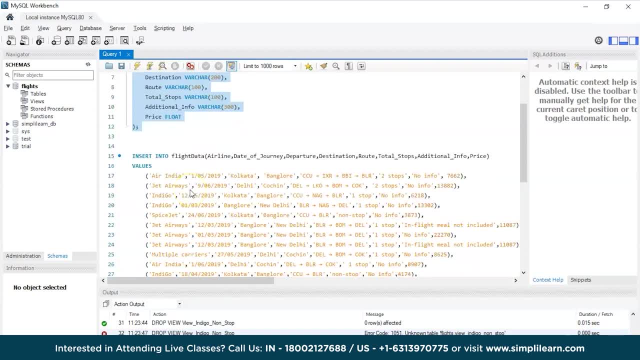 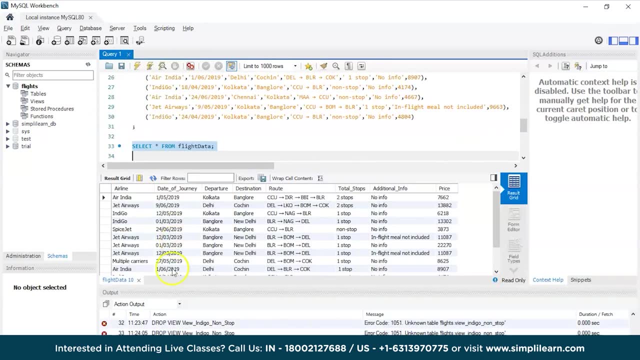 And in that we have a table by the name flight data And this is the data which we have added into a flight data. Right, Let's run this and get the table. So here you have the information on your table about a few flights. You have the airline date of journey, departure destination. 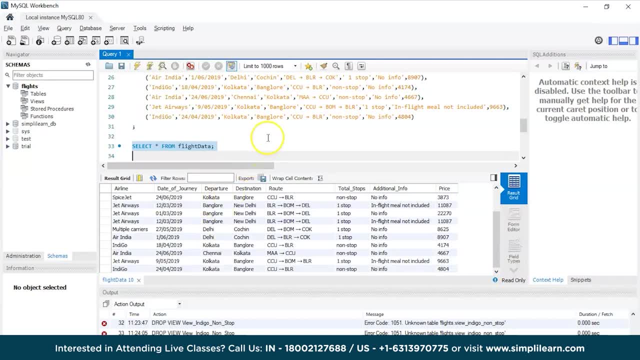 total stops, additional information, et cetera, et cetera. Right Now, let's say, if someone asked you to fetch a flight from Indigo which is completely non-stop control, enter Now you have this. Right Now, you face this query for once. 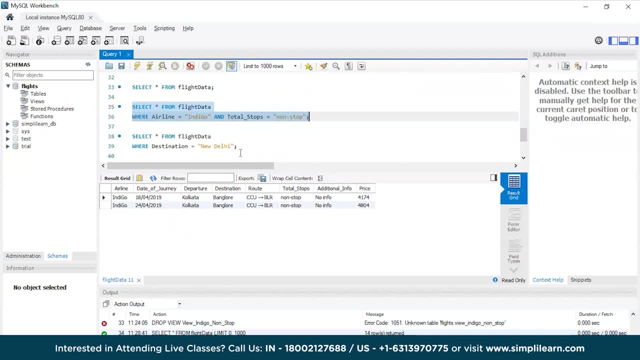 And what if someone asks you to get this data for 10 times a day? Maybe you have 10 clients who are asking for the same information. Would you write the same query 10 times? No right. Similarly, here you have, let's say, someone wanted to go to Delhi and they asked you to get the. 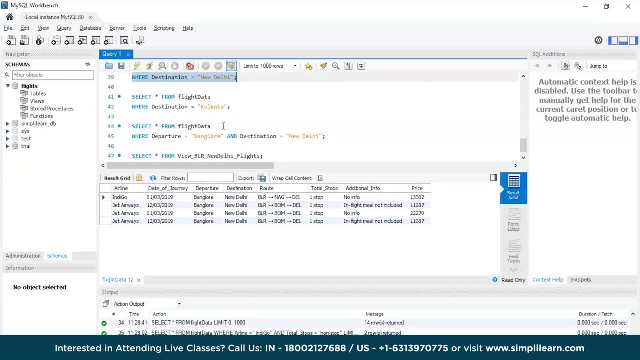 information for the flights which are going to Delhi, And someone asked for the flights which are going from Bangalore to Delhi. Right, Similarly, you have many of such things, So what would be helpful here? So, let's say, you add one more query which reads as: create view: 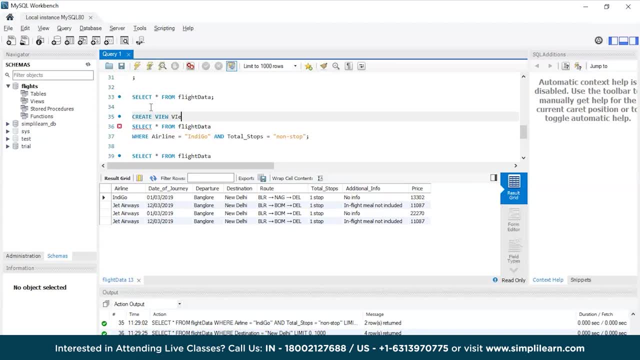 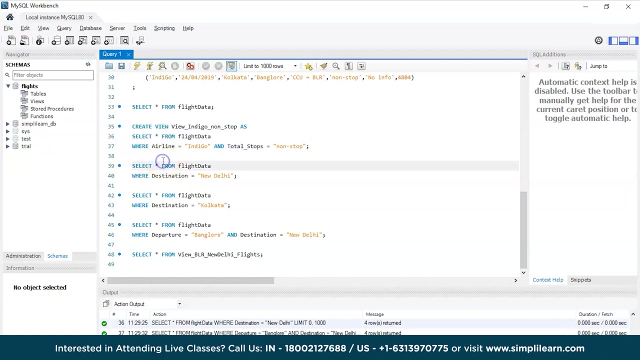 Now the customized view name could be anything. Let's say, view Indigo non-stop as your query. Right, Let's quickly execute this query and it should create a new view for you. The new view is currently done. Similarly, let's try to create a new view again.